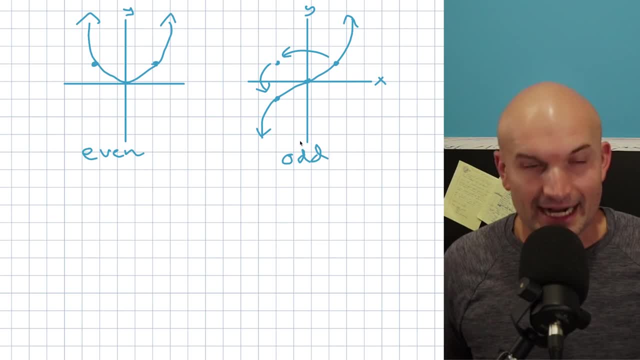 are reflected about the x as well as the odd function. so these are going to be odd. Now, this is why, if you understand the symmetry, this is also going to be why the algebraic approach kind of makes sense, right. So if I said like f of x, 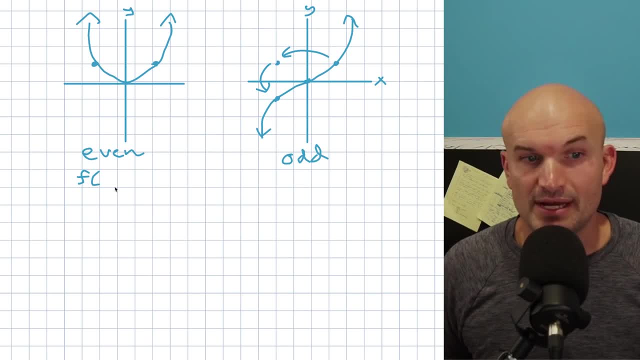 I'm sorry when we're trying to show if a function is, even algebraically, we say is f of negative, x is going to give you back the original function and again like kind of makes sense of this right. What if I said like here is negative one, right, and let's say I don't know, let's say this point is two. 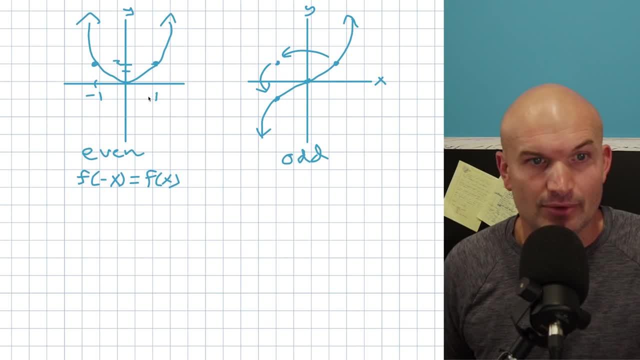 right. Wouldn't you agree that f of negative one is equal to f of positive one? right, They both have a value of two. so you can see how that kind of works, like f of negative one is two, f of positive one is two. See how, when it's reflected about the y-axis, that makes sense, Whereas an odd function it's. 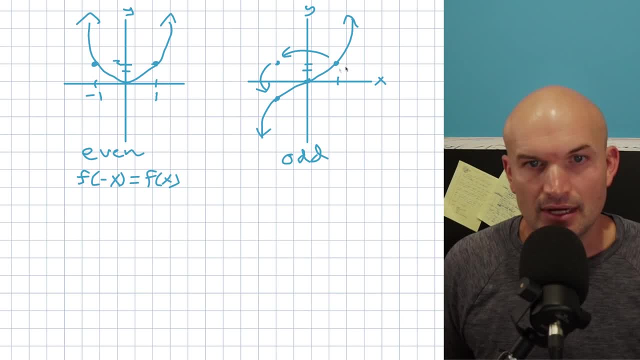 completely the exact opposite. Here's f of one right. let's say that's again two right. but then when I say what is f of negative one, you can see now that's going to be at a negative two right. So the definition for the algebraic approach, for showing that something is an odd function, you say: 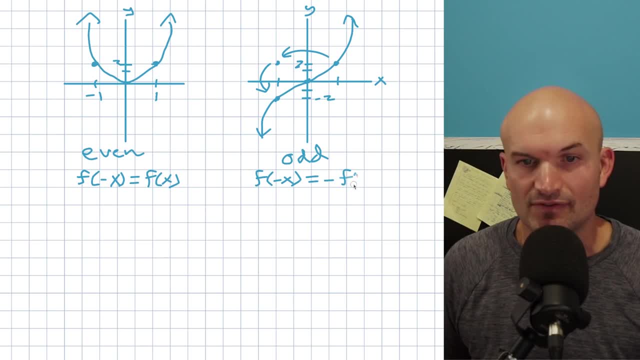 f of negative x is going to equal the opposite of your function, f of x. So what are some kind of tips that you can recognize? Well, I think the first thing that you should recognize if you're trying to identify if a function is even or odd, is just to graph it okay, and then look for symmetry. 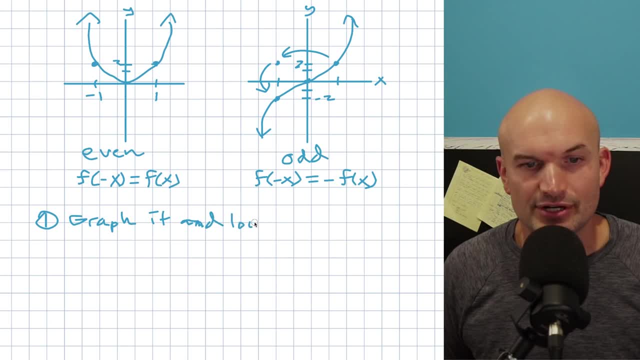 So graph it and look for the symmetry right. because, again, if you remember that if it's even, it's reflected about the y-axis, if it's odd, it's reflected about the origin. then therefore, you can go ahead and confirm just by the symmetry if it's going to be even or odd. Now the next step I want. 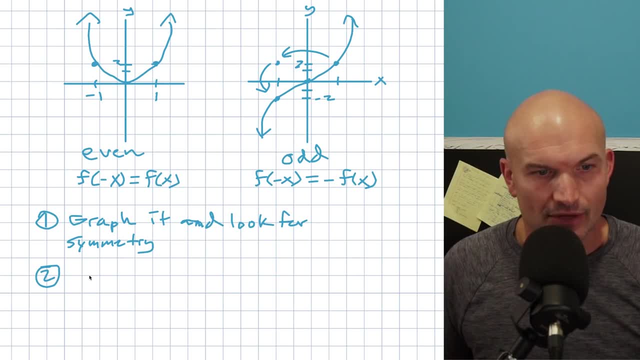 to do is really going to kind of focus on polynomials okay. So let's say I'm going to do a look at this and I say five x to the fourth minus a seven x squared. Now here's a polynomial okay, and one of the most common mistakes that students do when they're dealing with looking at polynomials. 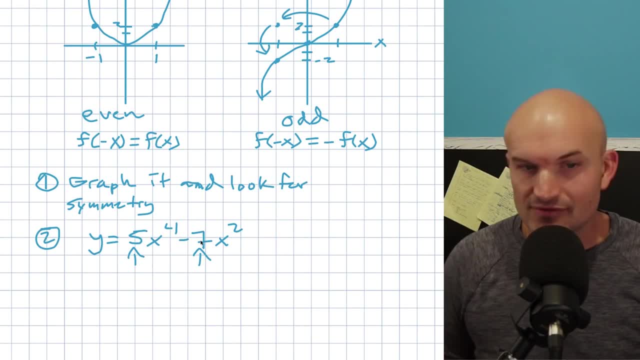 is they kind of focus on the coefficients. Do not focus on the coefficients. What you need to do is focus on the powers, all right. So what I want you to do is just kind of say: focus on the powers. Now there's a couple tips that I want you to do when you're trying to focus in on the on the powers. 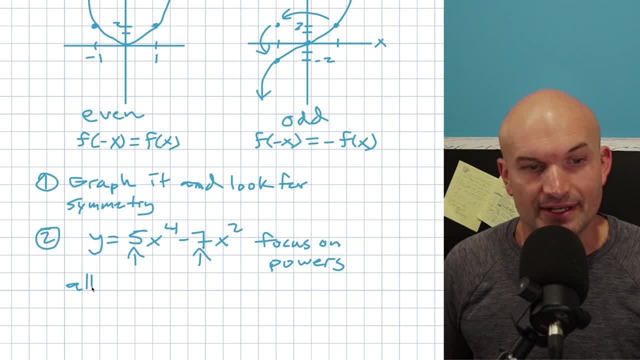 Okay. and when you want to focus in on the powers, what I want you to do is: if they're all even so, that means, like, you have x to the fourth, x to the eighth x squared right. if they're all even, then you have a even function. Okay, so you can see in this polynomial what do we have? We have. 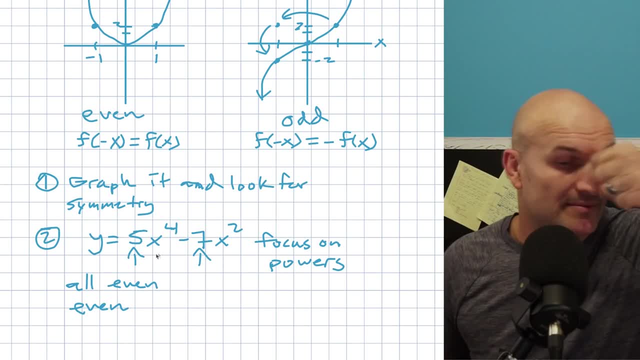 all even powers. Do not worry about the coefficients. We have all even powers, So therefore we're good to go right. So therefore that's an even function. So if they're all even, it's an even function. If they're all odd, right. so if you have x cubed plus x whatever, everything like that, then it's an odd. 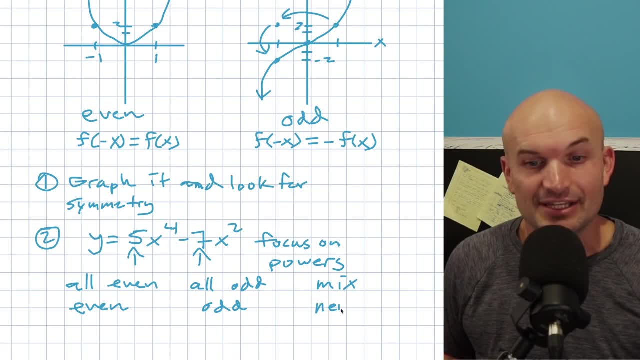 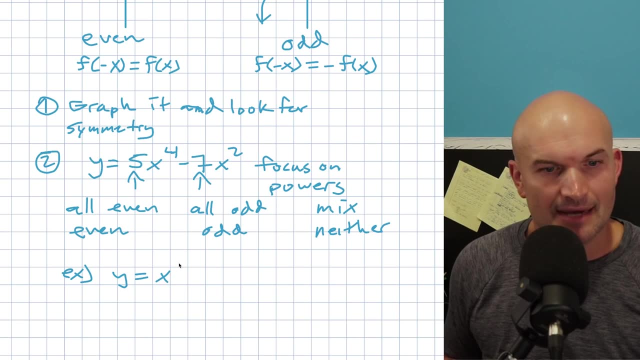 function, And if you have something that is a mix, well then that is going to be neither even or odd, right? So again, just kind of like a quick little example here: What if I did like a y equals x to the fifth plus x squared? That is not going to be even or odd. You can see that one is odd and one. 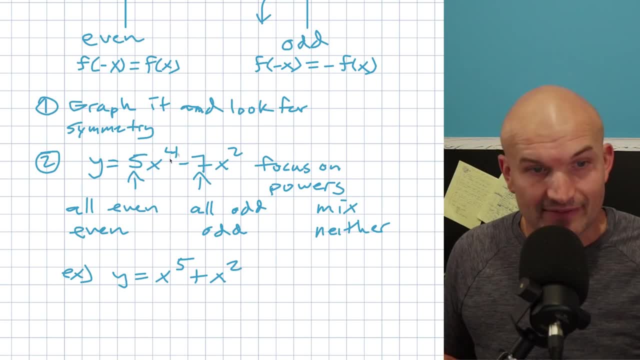 is even right, So it's not going to work. So it's either when the powers are all even, it's even, or when they're all odd, it's going to be odd. So that's kind of like a nice humble tip. And then 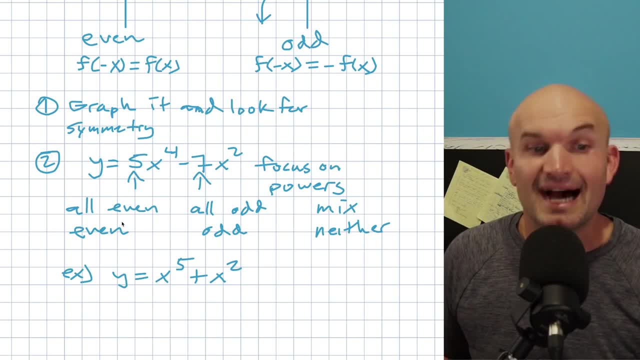 the last thing I always want to mention to you is also with the, with the constant. Okay, You could have all, even, all, even functions, and then you can have plus c, And what I mean by plus c is you can have a constant and the constant is not going to impact that. However, when you have 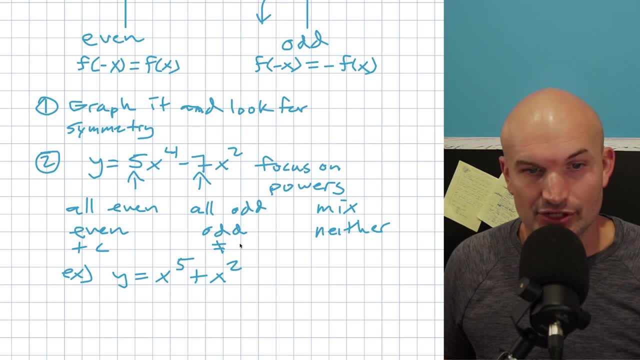 an odd, you cannot have c, Okay. So you cannot have a constant, You cannot have a number at the fact. So what I mean by that is like, for instance, if I say a y equals x cubed plus one, That is neither. 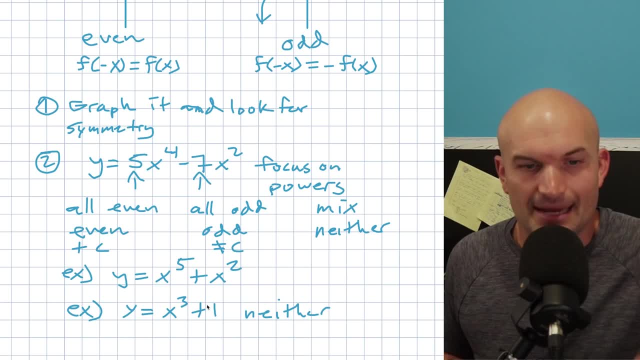 Okay. So a lot of students will get confused with that. They're like: oh wait, all the powers are odd, Yeah, But you have this constant here. It doesn't work when you have a constant, So you have to be very, very careful for that. 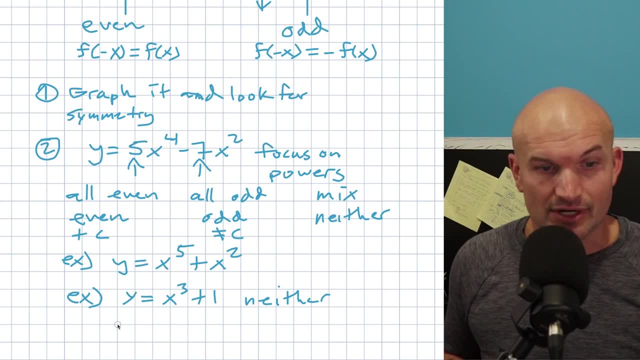 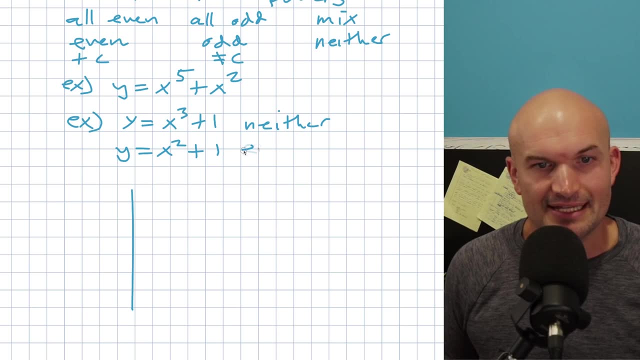 It would work for an. even So, if you have an even function and a- c like that works, y equals a, x squared like plus one That works. And again, like: if you want to see this, like, just go and take a look at that, That is even Right. And again, let me show it to you. Here is: let's take my quadratic. 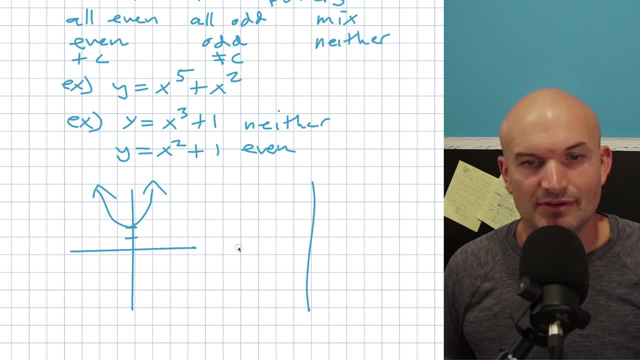 here You can see that's still symmetrical about the y axis. However, let's go and take the cubic function here and move it up one And you can see that now that graph, when you reflected about the x as well as reflected about the y. 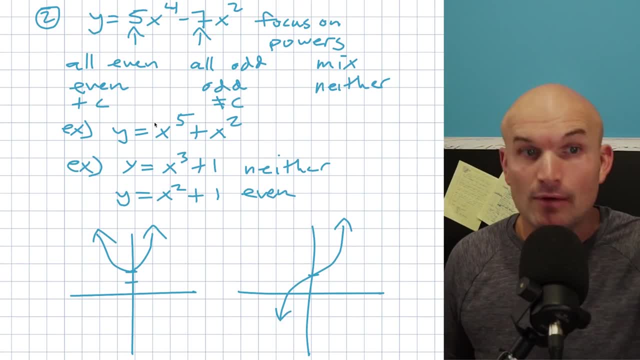 It's no longer even Right. So be very careful with the constants. They work when you have all powers are even. They do not work when you have all powers are odd, And no matter what, if you have a mix of evens and odds, they're not going to work. Okay, The next thing that I want to kind of 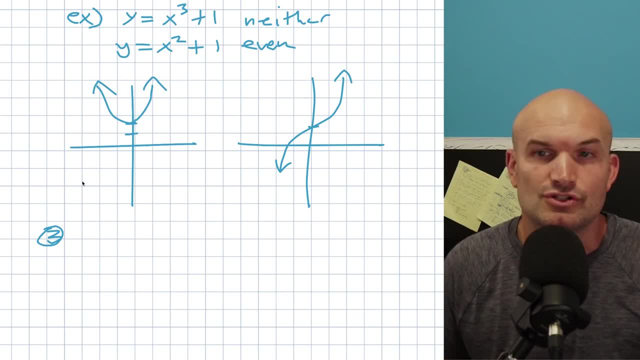 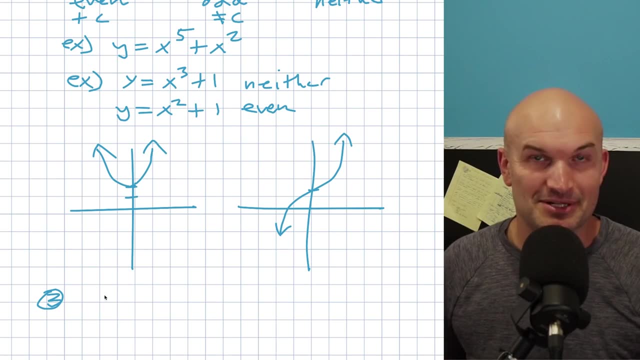 focus in with you is going to be when you have horizontal transformations. Now, horizontal transformations do not work very well, Okay, So when you have horizontal transformations, be very leery, And the two, the two most common horizontal transformations I would work with would be like when you're dealing like with an absolute value or like a 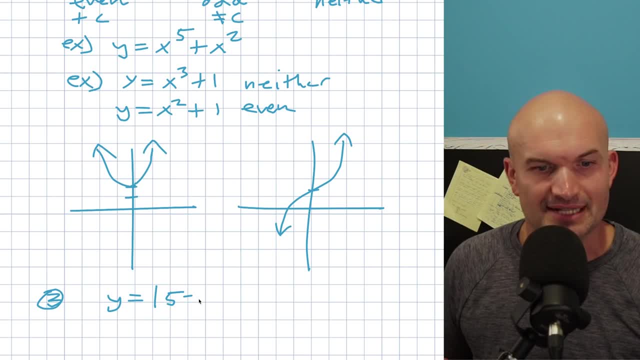 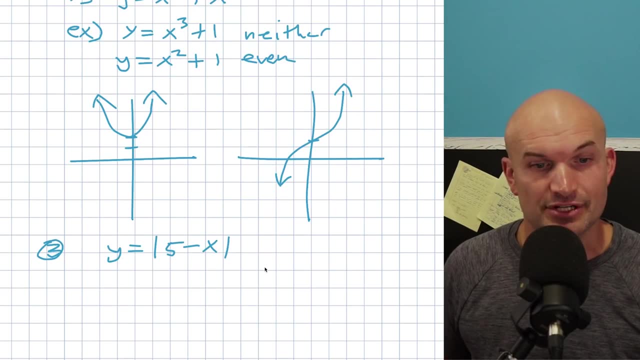 or a square root function. Okay. So if I had like five minus x, Well, let's just deal with the absolute value here. So five minus x. Now, this is not going to be an even, nor is it going to be an odd function. Now, typically, the absolute value function is an even function. Right, But what? 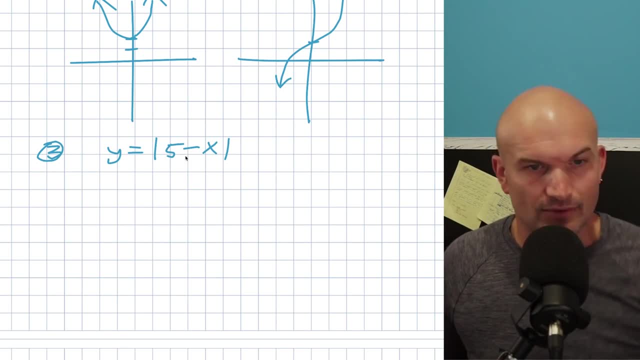 happens is this graph is shifting it. what you're actually reflecting about the y axis Right, And then plus, and then you're minus. you're shifting it five units to the right. So this graph actually has one, two, three, four, five. That graph is not reflective about the x nor the y axis. Okay, So. 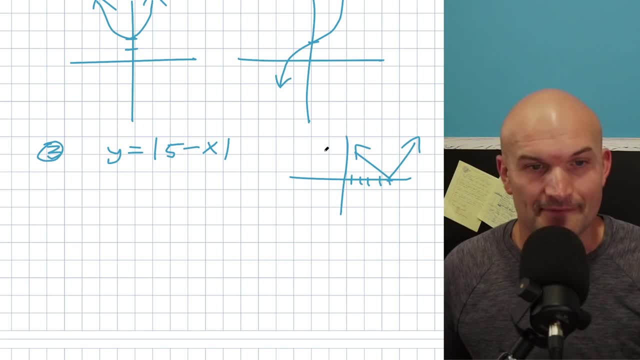 when you have horizontal transformations, you got to be very, very careful. like that's not going to work. The other reason why the horizontal transformations don't really work so well is you can't factor out a negative for the horizontal transformation. So let me show you. 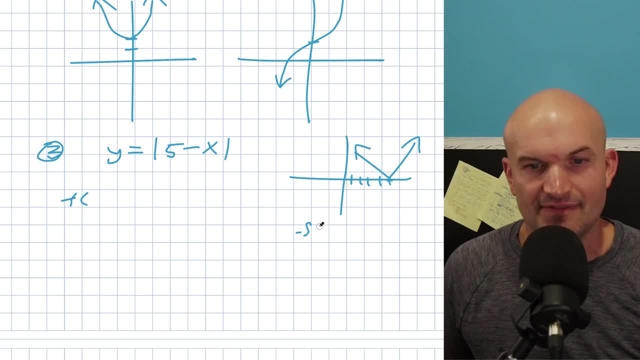 what I mean by that. If I had a function like- let's kind of put an example here- If I had f of x, Right, And I said, let's say my function is going to be a x cube Plus x, Okay, And if I want to say, hey, is this even or odd? Well, what would you do? You would 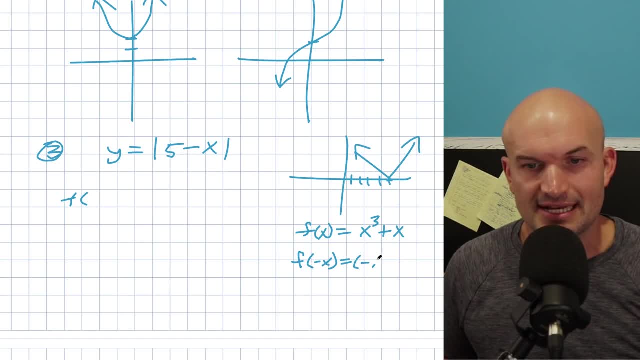 plug in a f of negative x, And when you do that, what you get is a negative x cubed, you know, plus a negative x. All right, So there you go. Then you just go ahead and simplify this and you say, all right, that's going to be a negative x cubed, minus x, And you might not be sure is that the? 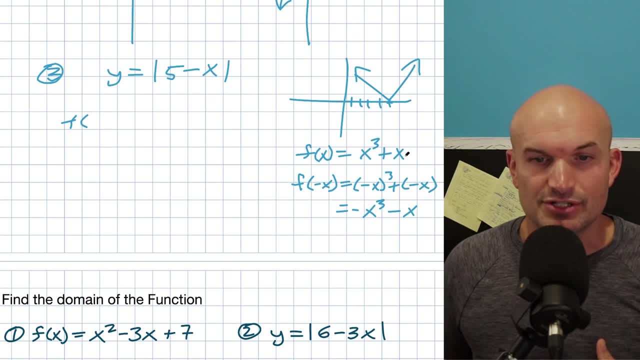 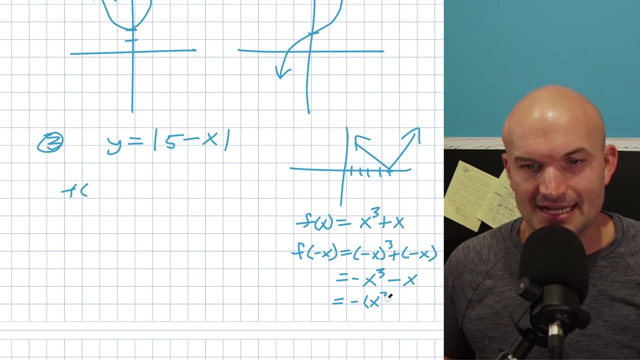 opposite of my function or not? And so what to do for that case? what you're going to want to do is you're actually going to want to factor out a negative. So when I factor out a negative here, say x cubed plus x, And what I want you to see here now is that is the opposite of f of x. Right, 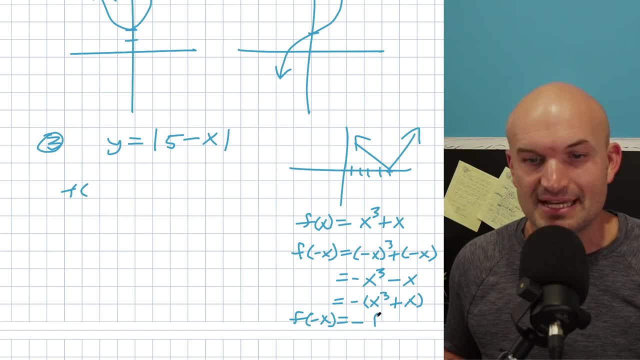 Now I can say f of negative x equals the opposite of f of x Right, Because it wasn't my original function: x cubed plus x Right, It's just the opposite of it. So therefore, this is an example of odd. So when you're trying to verify something as being odd, you've got to be, you want to be able. 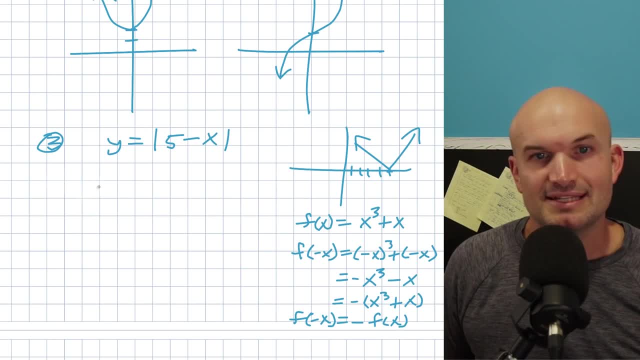 to factor out the negative. So that's why this comes in, That's why this is, when you have horizontal transformations, that's an issue, Right? Because, again, let's just try to rewrite this as a function. So let's say I had f of x, Right? So I'm going to try to verify something as being odd. 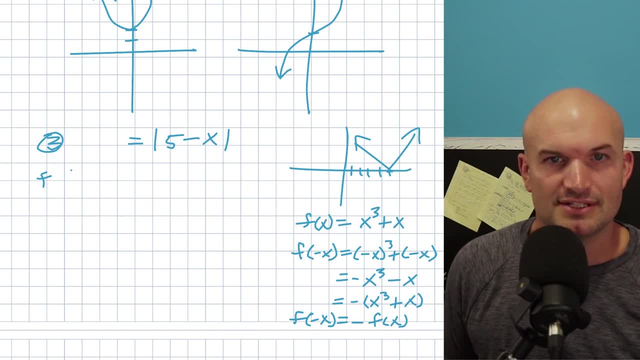 Or let's say, I wanted to test this, All right, So let's actually call this an fx. So let's say, all right, let's call this a function fx. So if I wanted to test f of negative x here, All right. 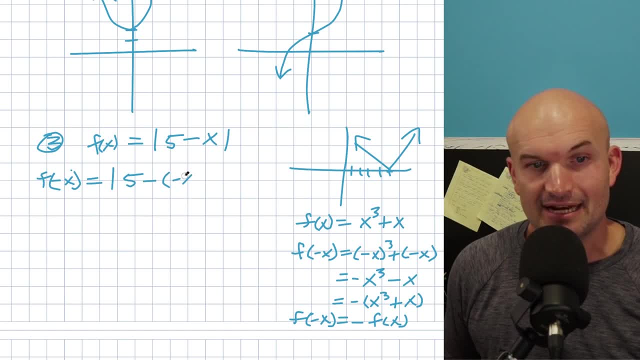 That's going to be absolute, absolute value of a 5 minus a negative x. Now we can go ahead and simplify this. Right, That's going to be a x plus 5.. Whatever, That's going to be fine. Like you can rewrite it, rearrange it, It doesn't matter, Right, It is 5 plus x, I don't care, Whatever. 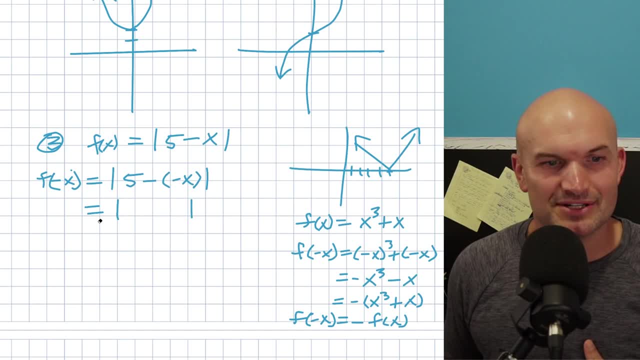 you want to do. The problem is, though, here's what I want you to see. So let's say, this is a 5 plus x. Right, So it goes minus a negative x. Right, It's 5 plus x. The problem is, we can't figure out. 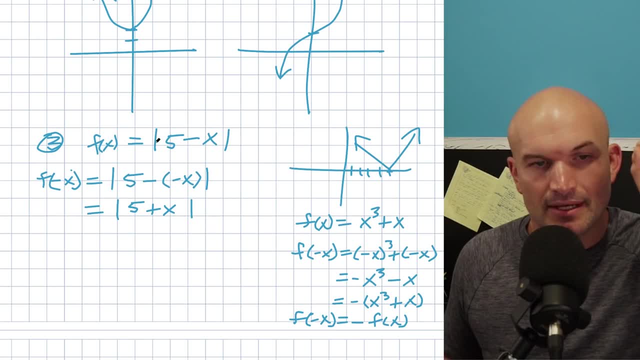 a negative. on the outside Right, F of x is a negative 5 minus x. So if I wanted this to be even, if this needed to be even, it needed to be a negative absolute value of 5 minus x. That is what would show as a odd function. I can't do that. You can't take a negative outside of like a radical. 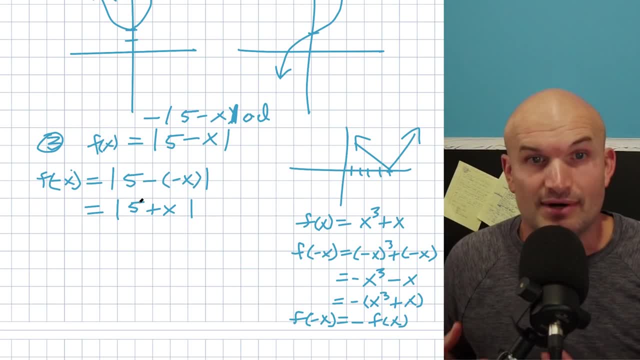 or outside of a absolute value, or outside, really, of any function. Right, You can't factor that term out. So the only thing you could do It was like factor out a negative inside, But that's not going to give you back your original. 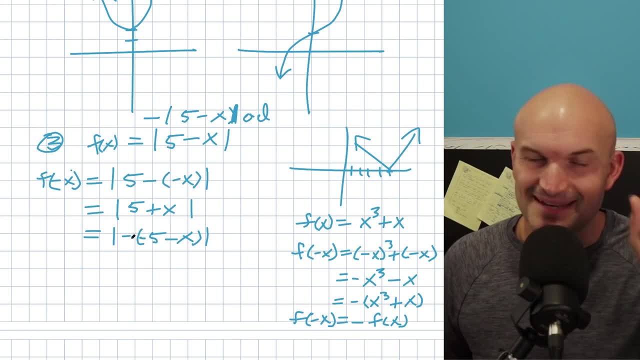 function, because actually, when you factor out a negative, that's a negative 5. Right, Don't make that mistake. So that's a negative 5.. So, therefore, this is neither. Now, I do want to give you some examples of how could we kind of rearrange this, though. so it would actually be an even, or it.